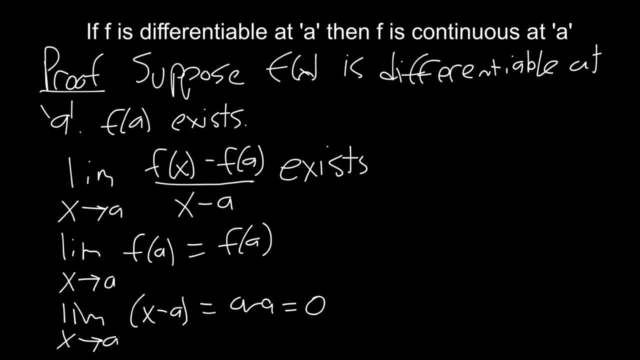 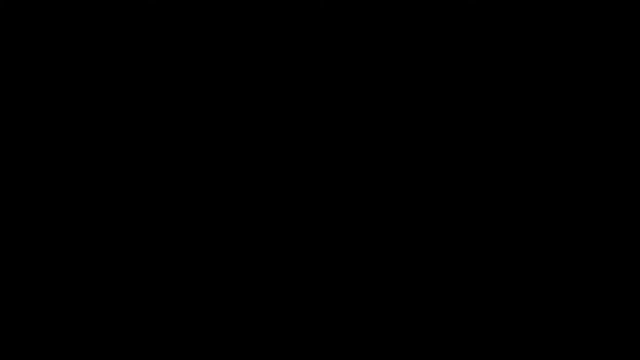 three limits that we know here and we need to combine these in some way to show that f is continuous. Now, to get there, we're going to have to rewrite f of x. So first we're going to rewrite f of x, as f of x is constant. So this means that f of x is nothing special. And if we write f of x as f of x, we're going to get f of x And this means that f of x is nothing special. So we're going to have to rewrite f of x as f of x is nothing special. 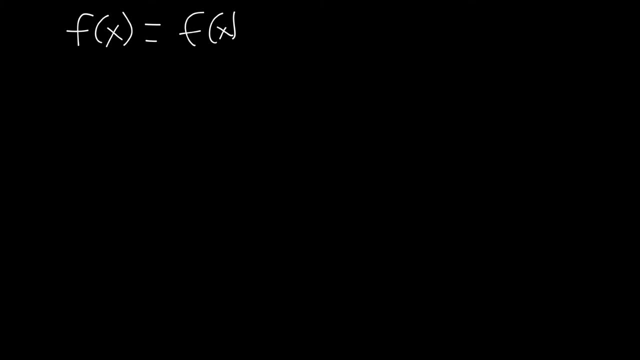 f of x equals f of x minus f of a, plus f of a. This is legitimate because we can add and subtract the same thing without changing f of x. Then what we'll do is we will take the first portion here: f of x minus f of a. 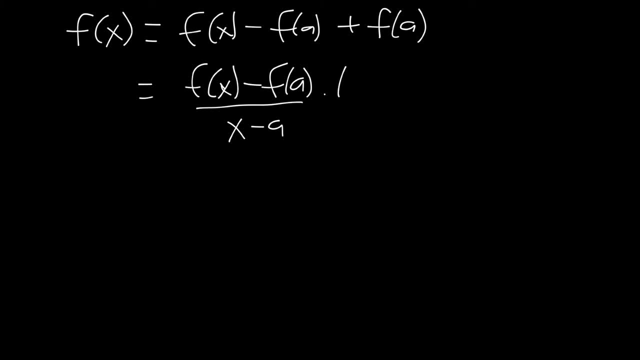 We will divide by x minus a and we will times by x minus a, still having f plus a at the end. So this is still equal to f of x. Finally, let's take the limit of both sides. So the limit as x goes to a of f of x. 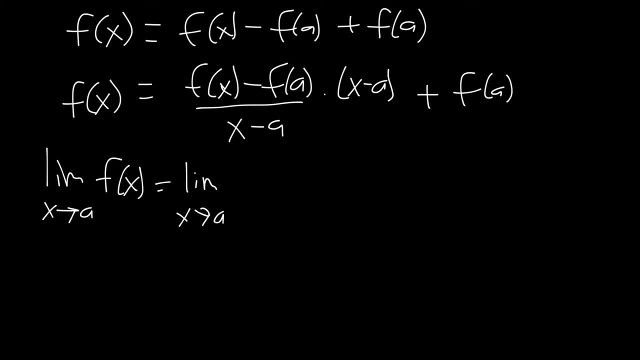 will equal the limit as x goes to a of the entire right hand side, f of x minus f of a. all over x minus a times x minus a plus f of a. Now, using the information we had from before, we know that this limit here, which 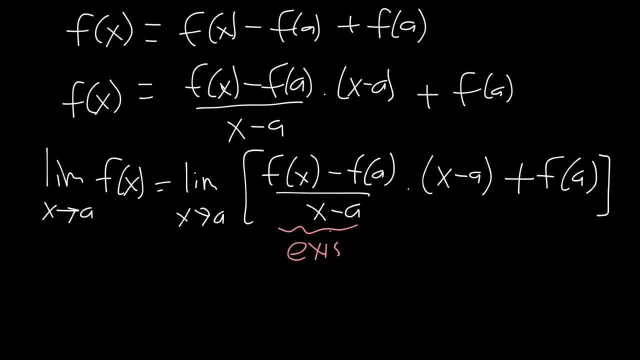 is just the derivative evaluated at a exists, This limit right here will be equal to 0 and this limit will be f of a. So, evaluating each part of the limit, we get prime of a times 0 plus f of a, which is just equal to f of a. so we can say that: 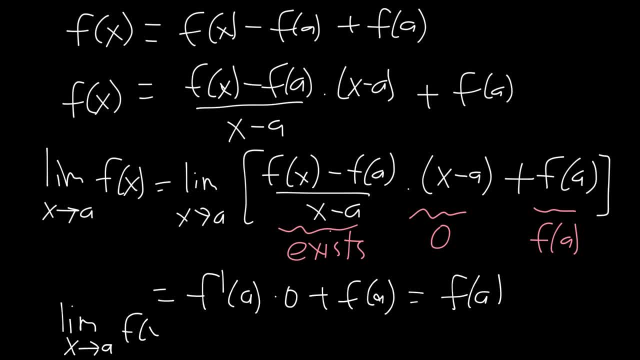 the limit as X goes to a of f of X equals f of a and f of X is continuous. and that concludes our proof. thanks for watching.